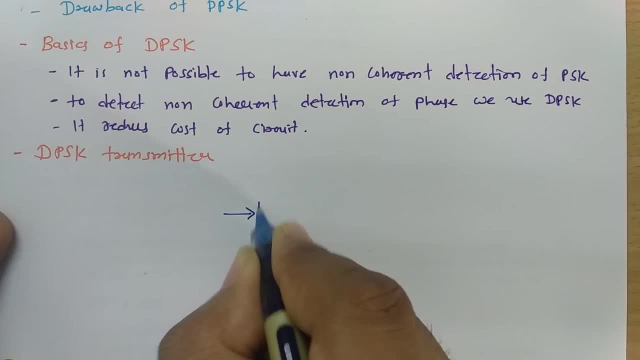 If you see, for PSK we were been having this type of block diagram. I think you might have seen that. If you have not seen that, you just go through my last session where I have explained this, where what I have done was we were been having message signal and that is what we are making it to polar waveform, and then we just multiply that with high frequency carrier signal. 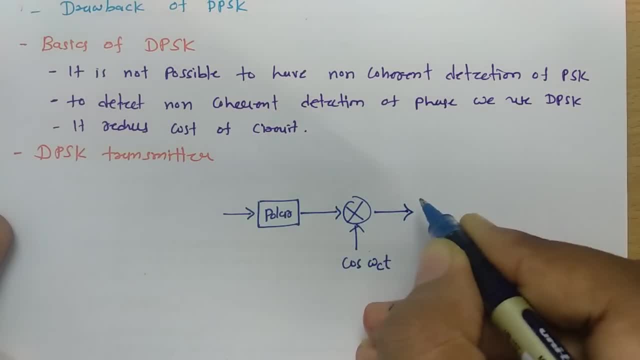 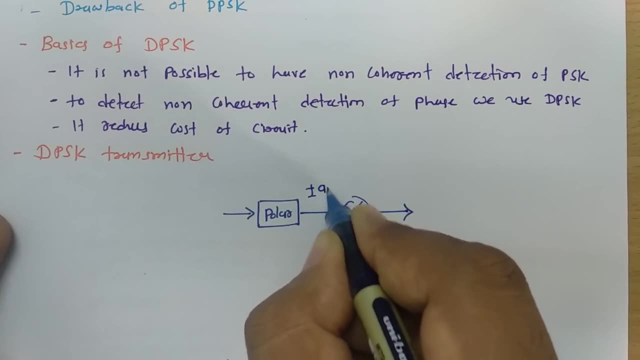 And that is what generating multiplication of these two. Now see, if I say, after having polar waveform, you have plus or minus AK voltage. For plus AK there is 1 and for minus AK there is 0. So if you multiply these two you will be getting plus or minus AK cos of omega CT. So that was the case, which we have seen it in PSK. But what is the difference in DPSK? 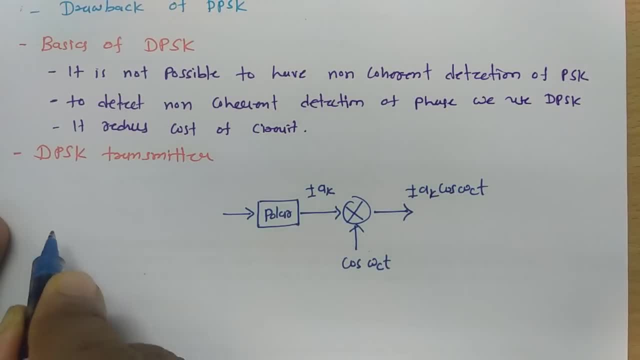 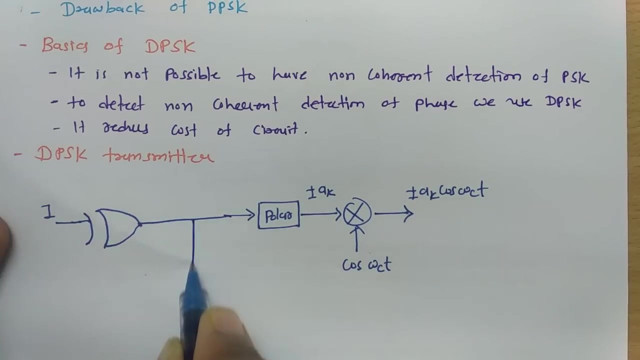 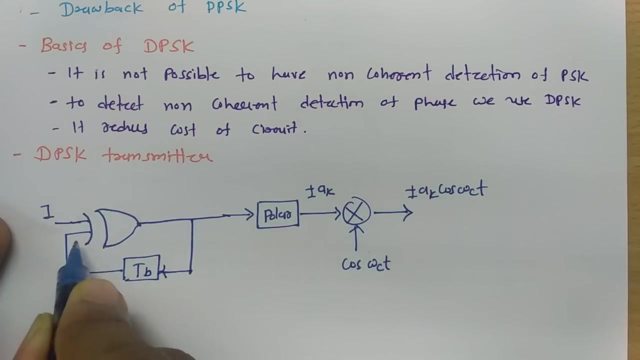 In DPSK we do is we take input. we take input and that is what we XOR. that is what we XOR with delayed output. so here we have 1 bit delay, here we have 1 bit delay. so all we do is we XOR input with 1 bit delayed output and that will be giving you phase change in between current. 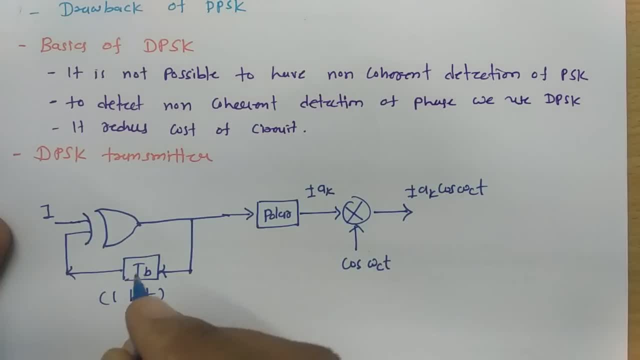 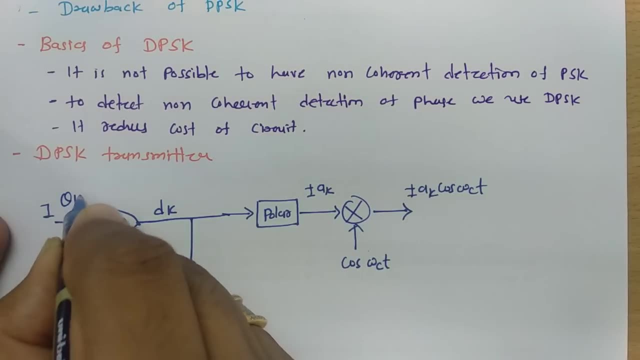 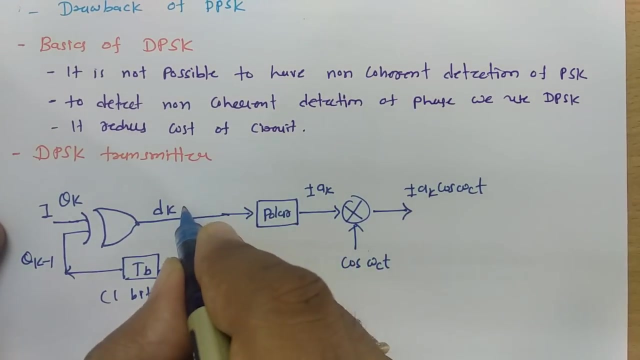 and previous bit. so here if I say I have this input that is D of K, and if I give current input that is theta K, then this delayed signal that will be theta K minus 1, so our D of K. that has to be difference in between these. 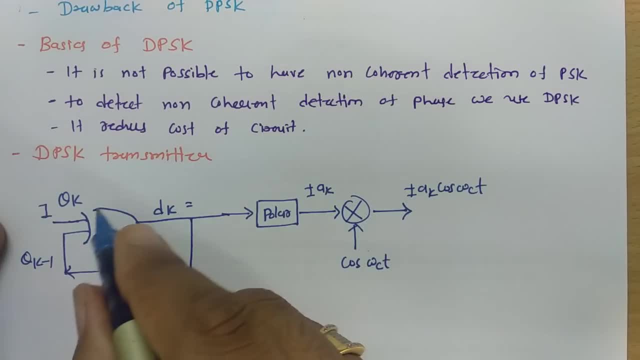 two, as this is what XOR, which is what product modulator- sorry, this is what XOR gate- that one can say it is modular to addition. so in modular to addition it will be taking difference of this two. if difference is there, then it will be giving you high if same signal is. 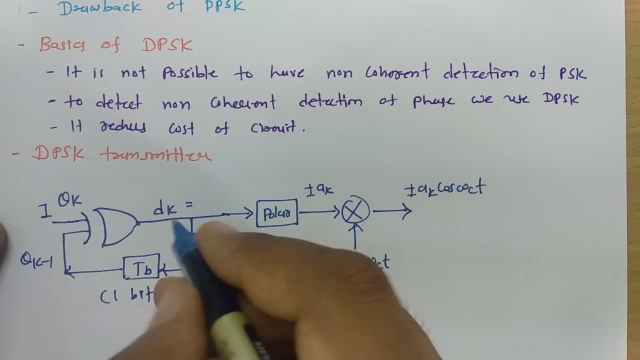 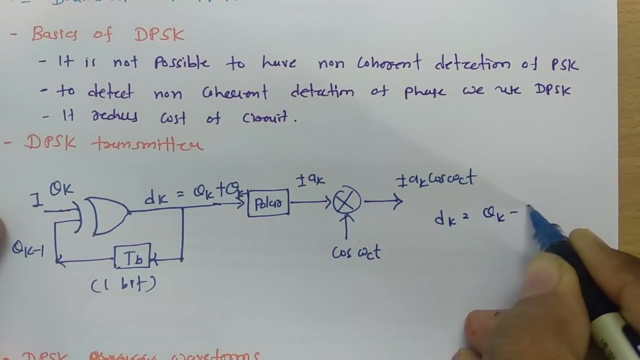 there. in that case it will be giving you low. so ultimately this D of K that has to be theta K plus theta K minus 1. so if you try to understand this characteristic D of K that is theta K minus theta K minus 1, what it means is it is XORing practically what 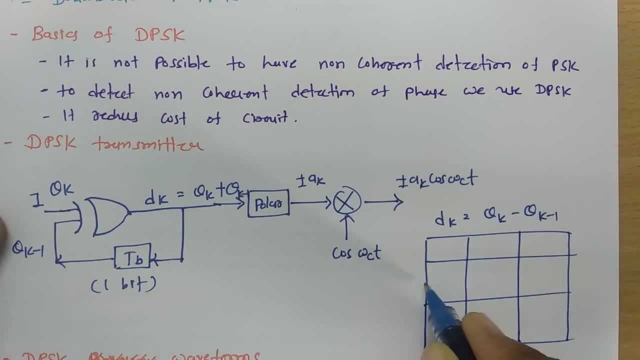 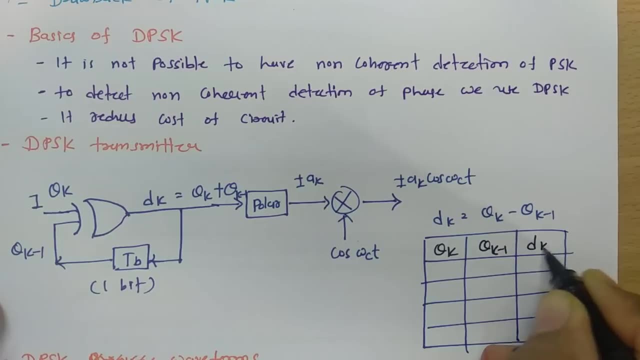 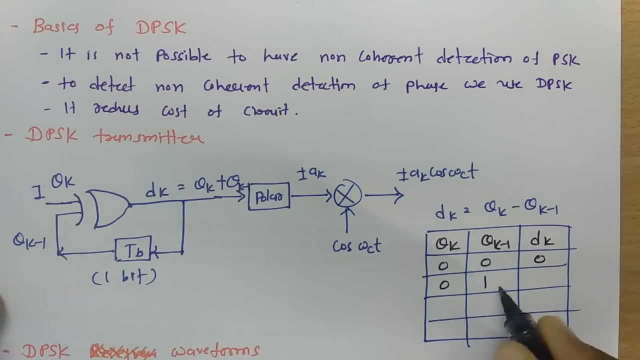 it means is it is XORing practically. And If I say here, this is theta K, this is theta K minus 1 and this is D of K. and if it is 0, 0, difference is 0, so D of K will be 0. if this is 0, 1, difference is 1, so D of K will. 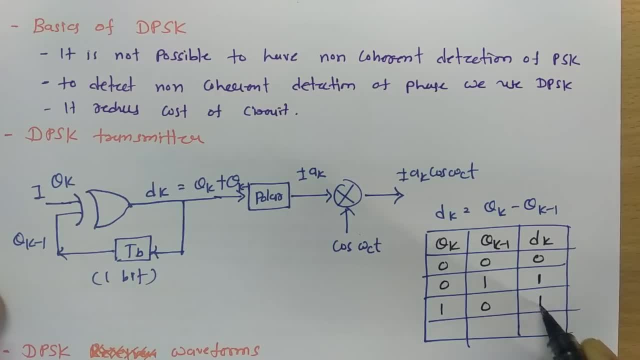 be 1. if it is 1- 0, difference is 1, so this will be 1. and if it is 1- 1, difference is 0, so output will be 1. so see, this is how difference that is been given by this XOR gate that is. 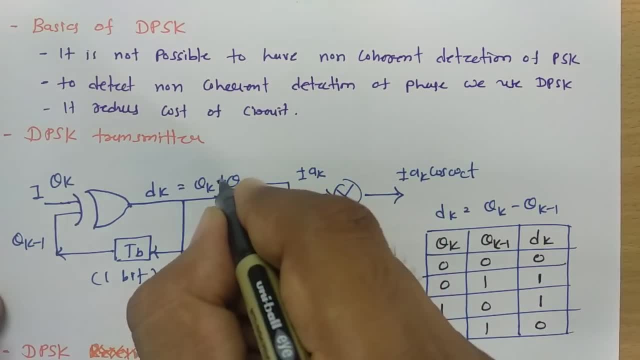 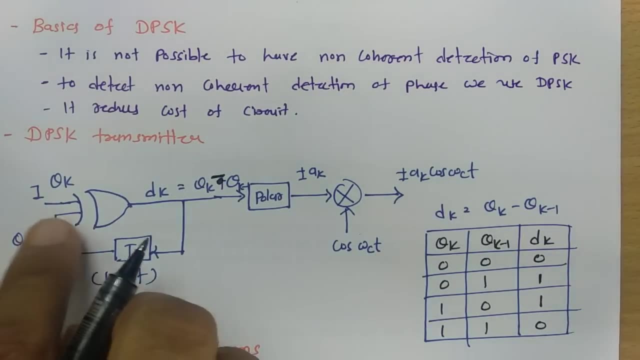 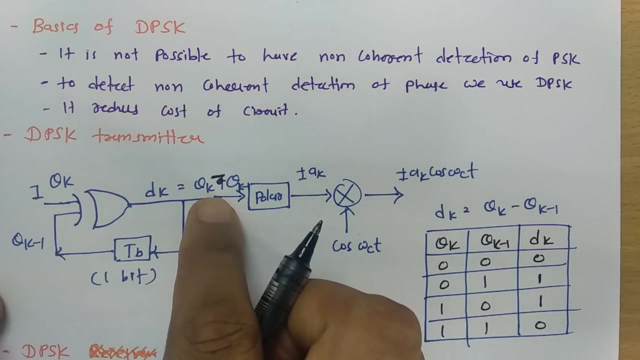 what D of K that is. That is theta K minus theta K minus 1. so that is how D of K is getting generated and that difference that will give you a phase in between current and previous bit. and when we give it to polar signal, it will be generating plus or minus a k amplitude. and when you multiply, 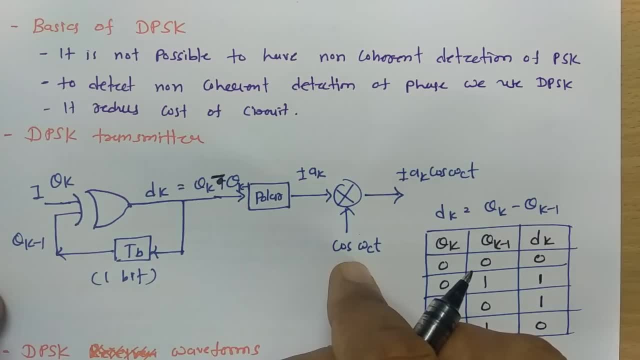 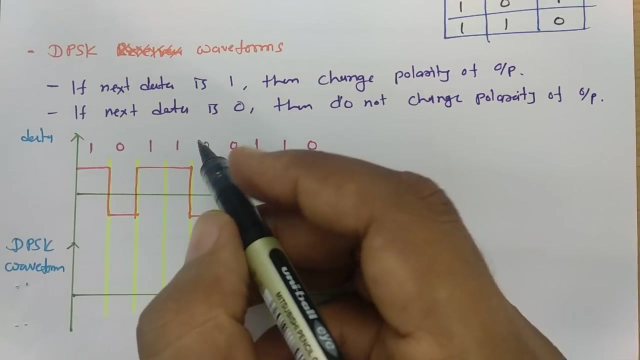 that with high carrier frequency, high frequency carrier signal, it will be generating plus or minus a k Plus of omega CT. Now let us try to understand how waveforms of DPSK that is getting generated. So see for that all we need to see is: if next data is 1, then there will be change in polarity. 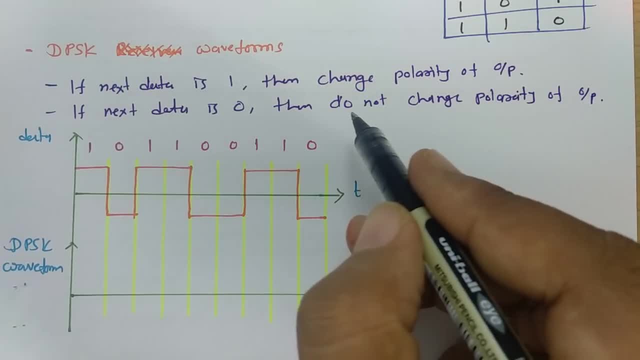 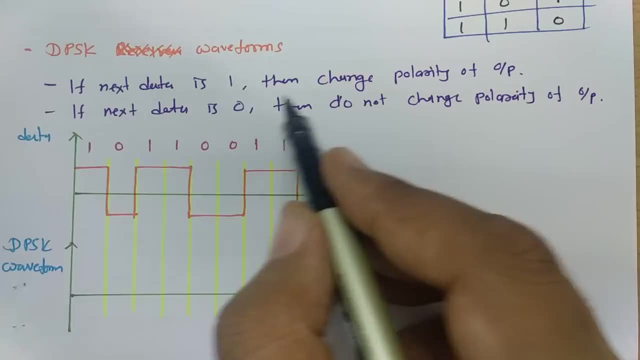 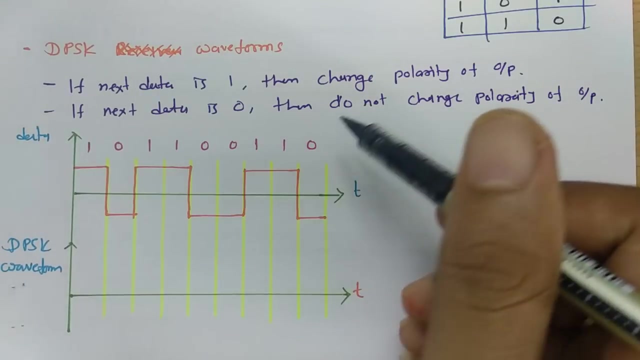 at output side. If next data is 0, then one can say you should not change polarity of output. So remember this: if next data is 1, we should change polarity of output if next data is 0.. If next data is 0, do not change polarity of output, and let us try to understand this with. 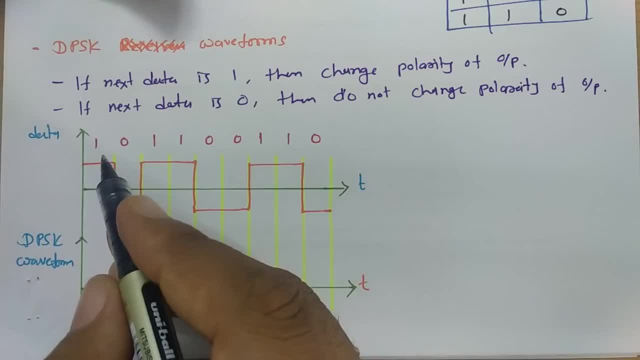 one example so it will be more clear. So see, here data is been given and that data is 1010. that one can see, which is written over here: for 1 it is plus amplitude and for 0 it is minus amplitude. So what will be our DPSK waveform? 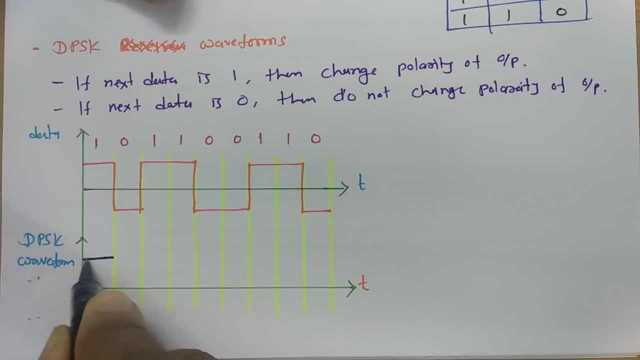 So see, initially there is one, so let us consider that one. Now see, as I have told you, if next data is 1, change output polarity. if next data is 0, do not change polarity. So next data is 0, so we should not change polarity of output. 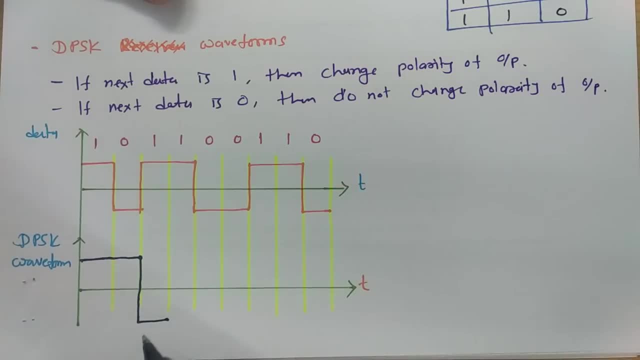 Next data is 1 here, so we should change polarity of output. so now it will be negative Again. next data is 1, so we should change polarity of output again. you can see polarity is getting changed. If next data is 0, do not change polarity of output. 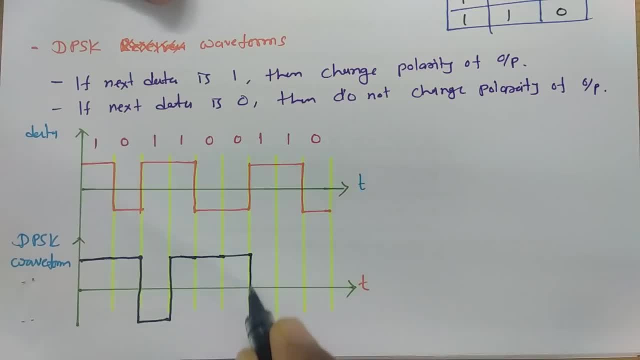 Again: 0. do not change polarity of output Again: 1. you should change polarity of output Again: 1. you should change polarity of output Again: 0. you should not change polarity of output Again: 0. do not change polarity of output. 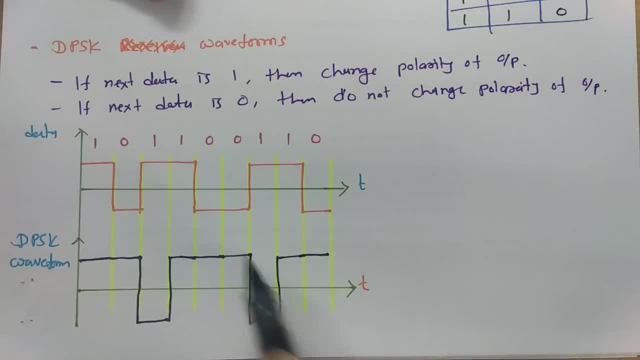 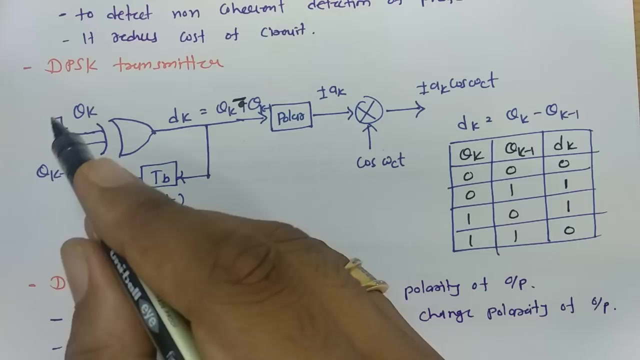 So see, this is how output waveforms that we can generate by using DPSK, where if next bit is 1, change polarity of output, if next bit is 0, do not change polarity of output. And again you see this DPSK transmitter where what all we do is we just XOR current bit. 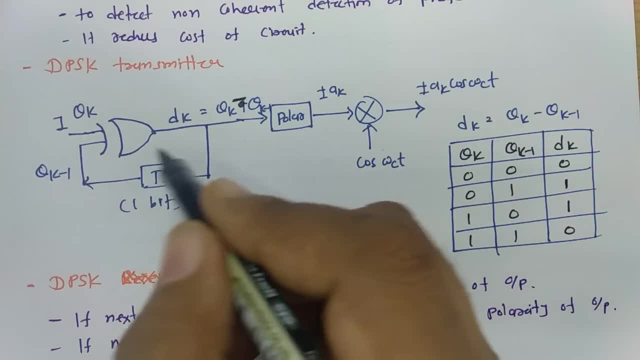 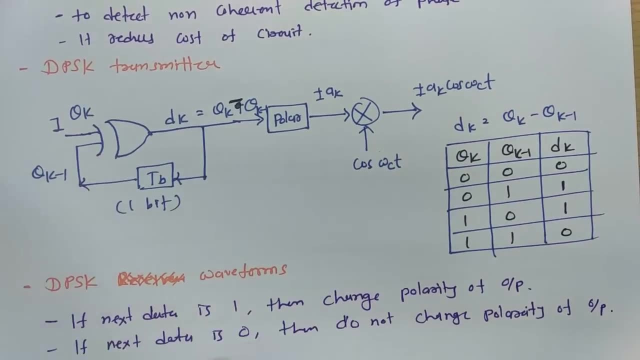 with previous bit. so we take one delay of 1 bit and XOR it and then you just do same thing as you do it in PSK. that will generate DPSK. Now I will explain you DPSK receiver, so it will be more clear. 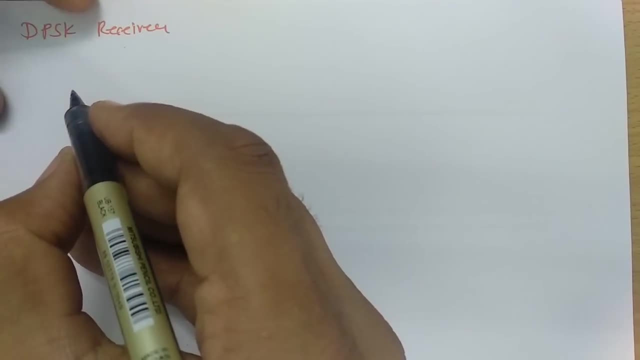 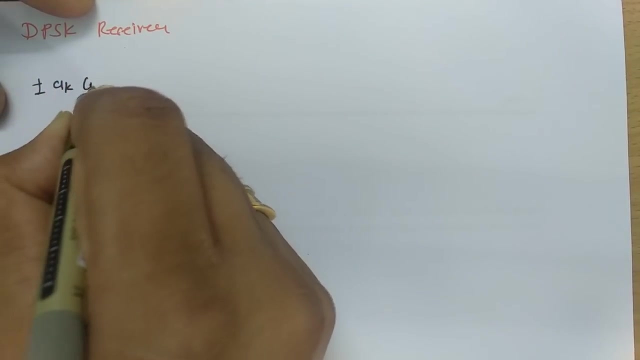 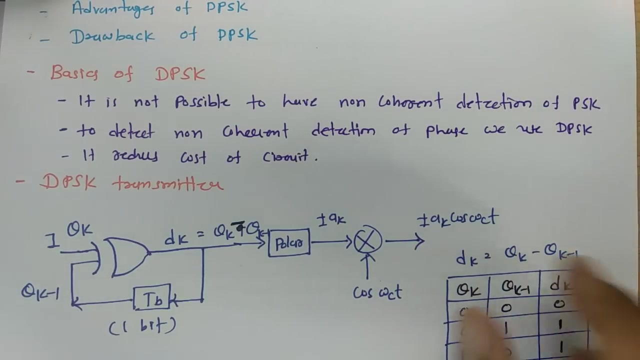 Now see, we just need to do exact reverse process as we do it in transmitter section. So here you have been receiving AK cos of omega CT signal. you can see what I have generated here, plus or minus AK cos of omega CT signal. So I have received same signal. 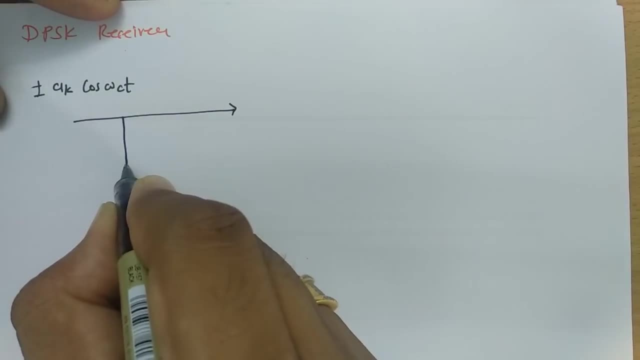 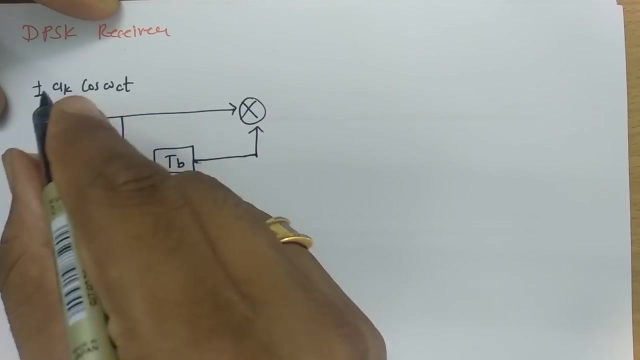 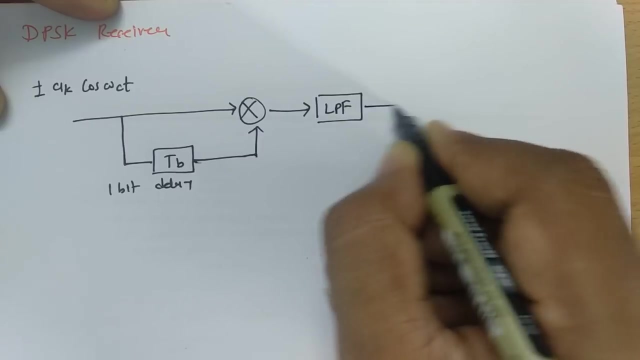 Now what I will be doing is: I will be, I will be passing through 1 bit delay TB and I will be multiplying this with this current signal and then, if I pass it through low pass filter, I can be able to generate output ZT. 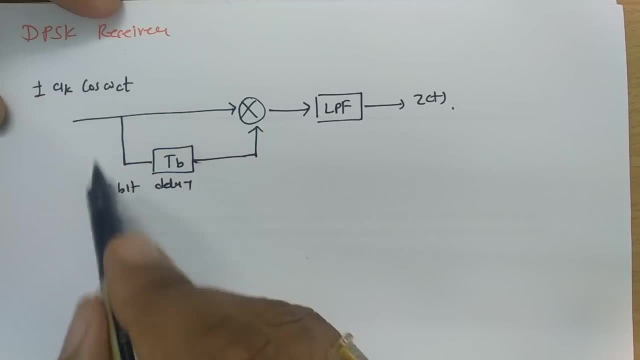 So see, all we do is we have received signal, Multiply it with delayed signal And then pass it through low pass filter. it will generate DPSK output. sorry, detected DPSK output. Now see how it will detect it. So for that I will consider 2 cases. 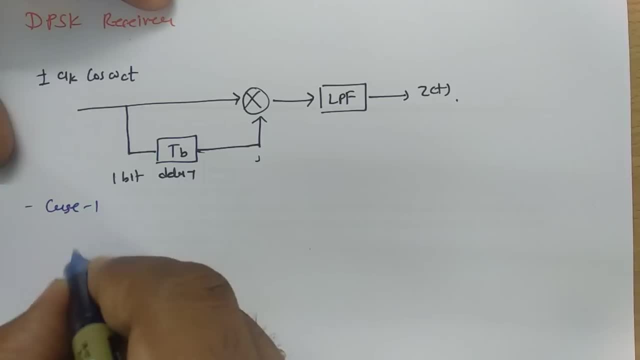 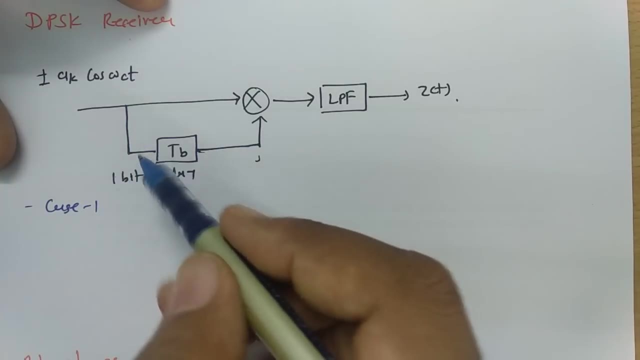 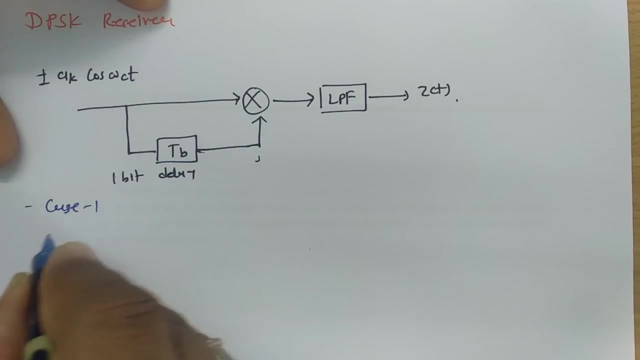 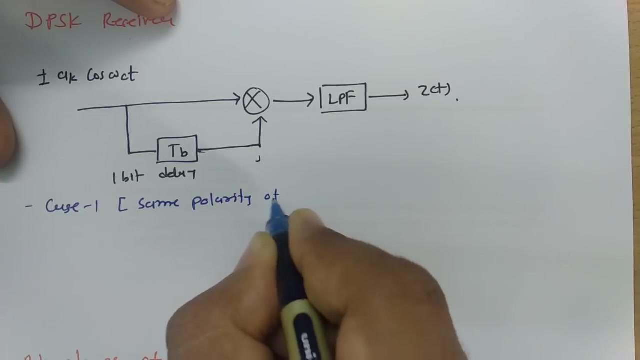 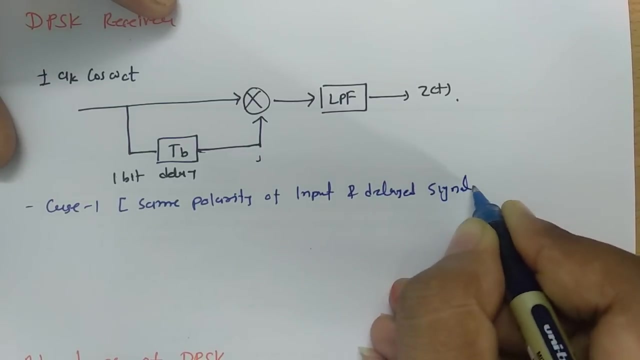 Now see in case 1, if I say I have received signal and both signals are having same polarity, I have received signal and both signal Like: see this signal As well as this delayed signal. Both are having same polarity, So same polarity of input and delayed signal. 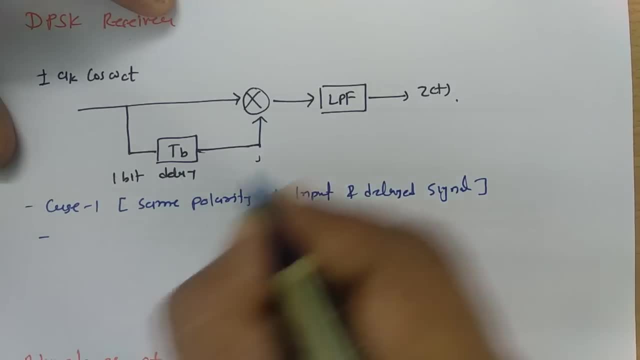 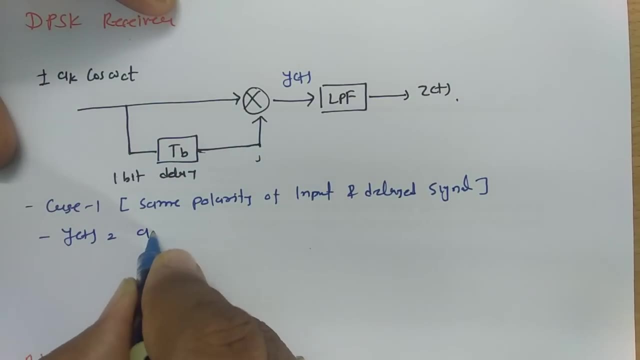 So let us consider first case. So in that case, if I say this is my YT, then this YT that will be multiplication of AK cos of omega CT. Same polarity means both are AK cos of omega CT. It could be minus AK cos omega CT, minus AK cos omega CT. 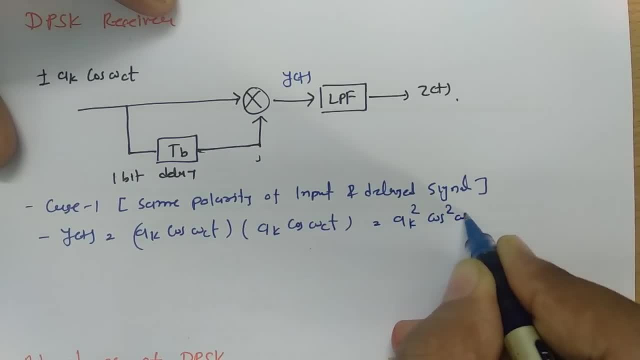 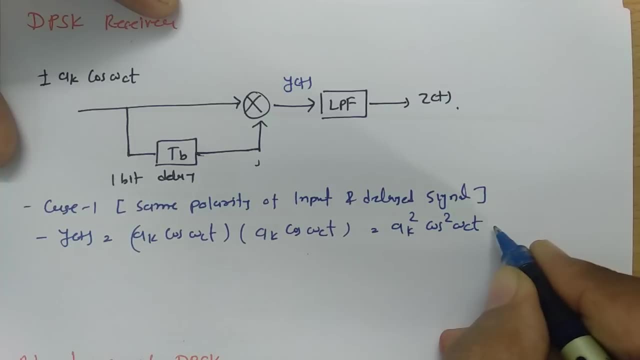 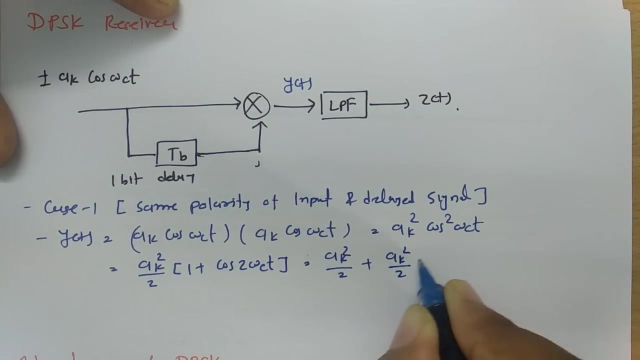 Multiplication, that will be AK square cos square omega CT. Now, if I re-elaborate this, then you will be finding: this is AK square by 2 into 1 plus cos 2 omega CT. So that is AK square by 2 plus AK square by 2 cos 2 omega CT. 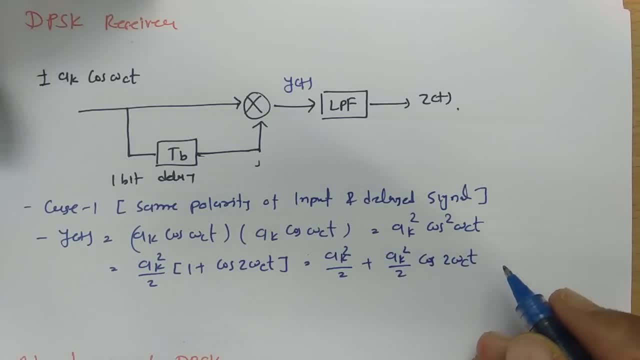 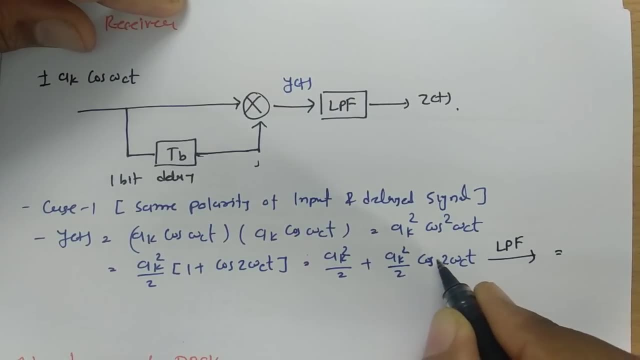 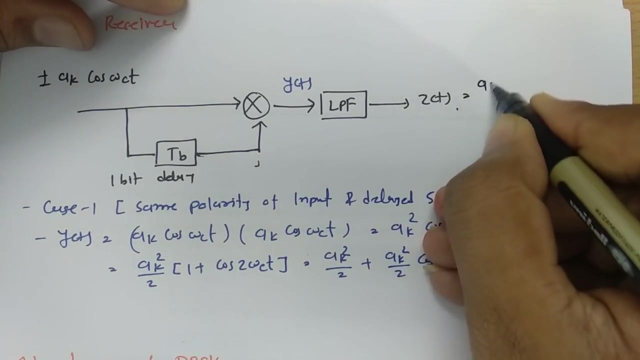 Now, when I pass this through low pass filter, When I pass this through low pass filter, you will be receiving. you will be removing this component, So there will be AK square by 2.. So here you will be receiving AK square by 2.. 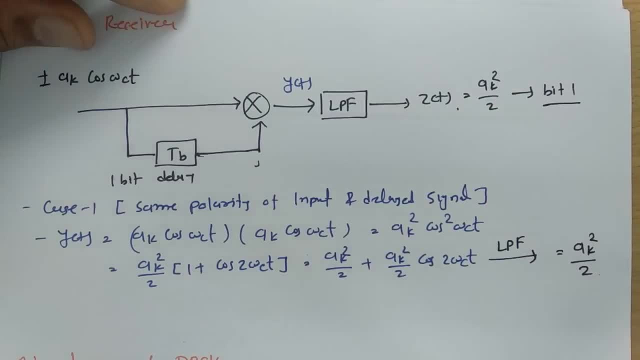 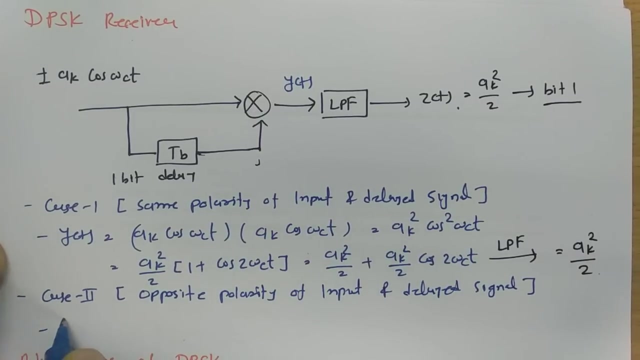 And that is representing bit, Bit 1.. So that is what the case which is happening here. Now let us have second case. So in second case, Opposite polarity of input and delayed signal. So in that, In that Y of T that will be AK, cos of omega, CT 1 will be positive and delayed. one could 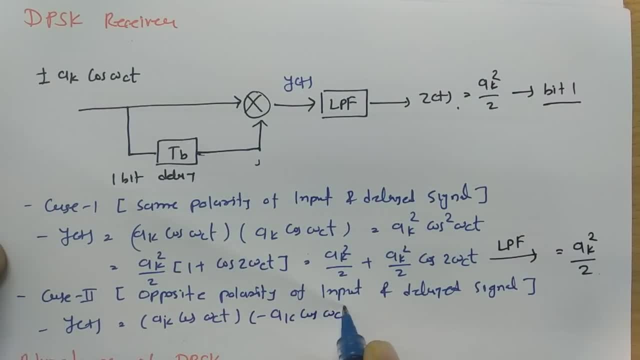 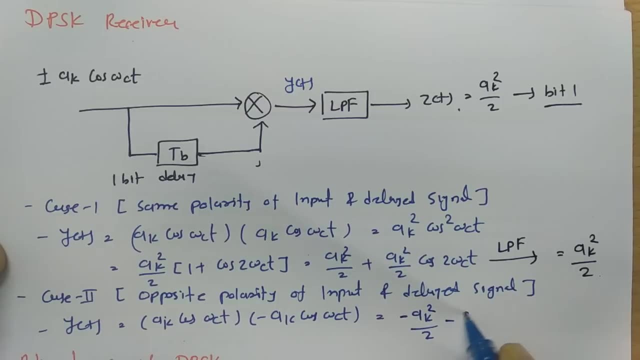 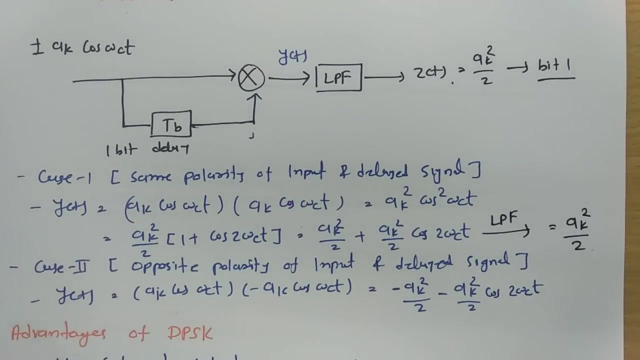 be negative, So minus AK cos of omega CT. So if you further calculate this, you will be finding it is minus AK square by 2, minus AK square by 2 cos of 2 omega CT. Now, as if you pass this signal through low pass filter.